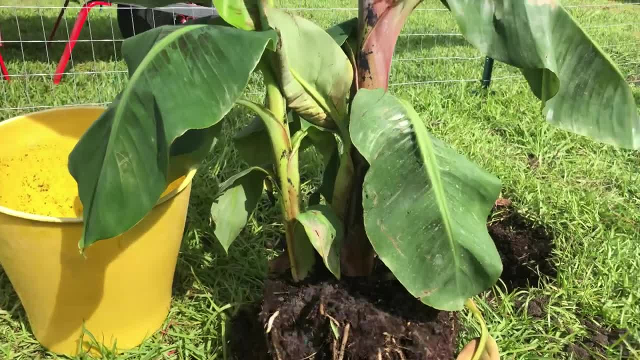 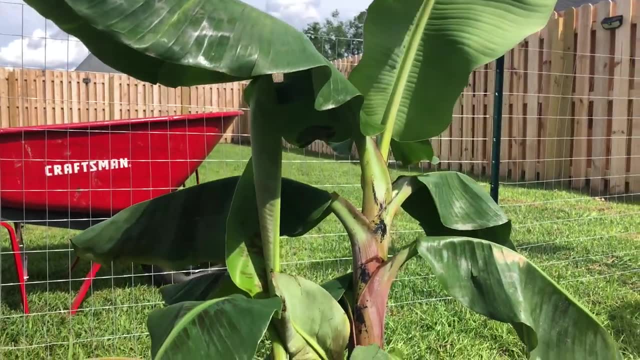 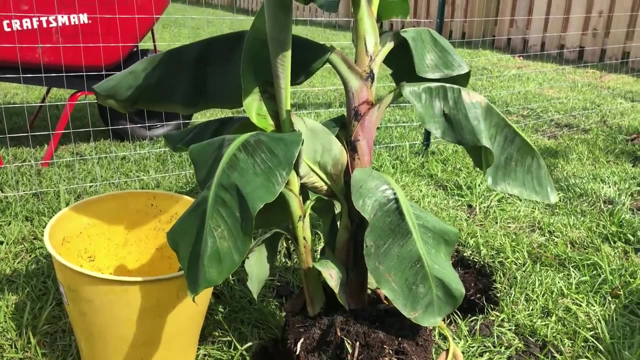 dwarf Cavendish. so, as you can see, there's actually a pretty large sized pup on this one right here. we're gonna go ahead and break that guy off before I put this one in the ground. my buddy Garrett- he lives in Atlanta, he's gonna take this one from me and he runs a cooking channel on Instagram, so he's. 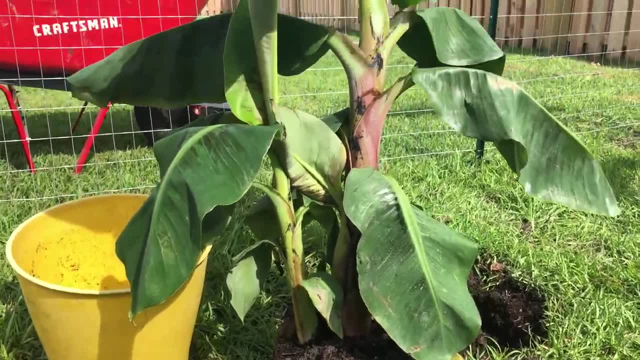 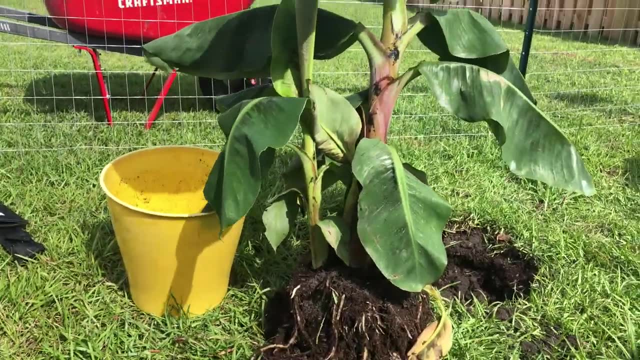 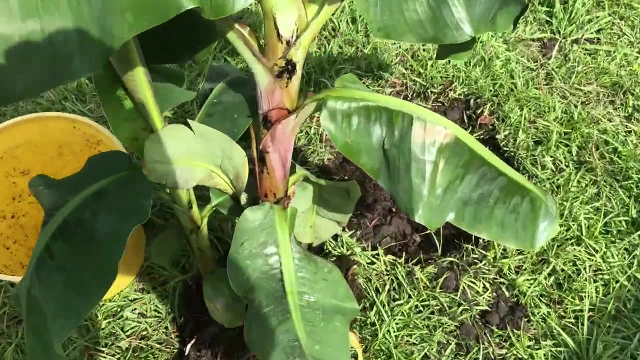 gonna make something with the homegrown bananas in a year or so. so I'm gonna go through the process of this. I showed it briefly in my previous video, but now I'm gonna go into a little more detail. so the banana tree: in themselves, they only fruit one time and so eventually they're going to grow up and they're going to 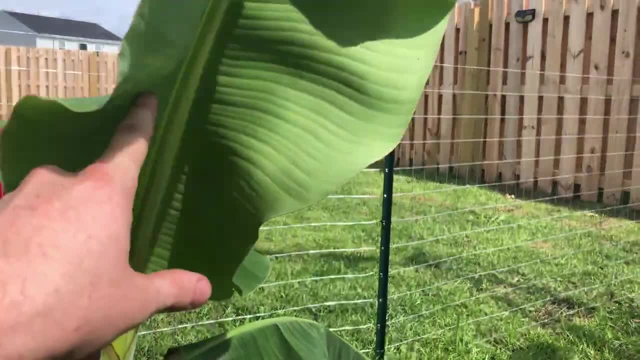 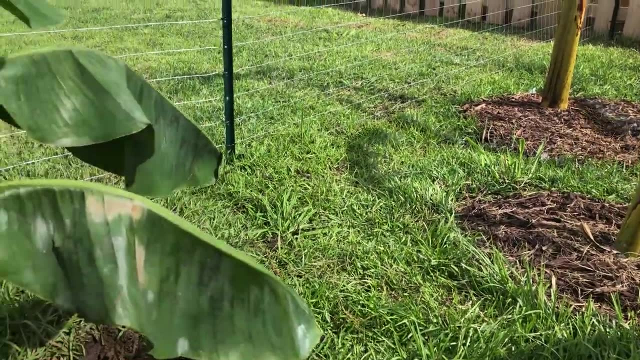 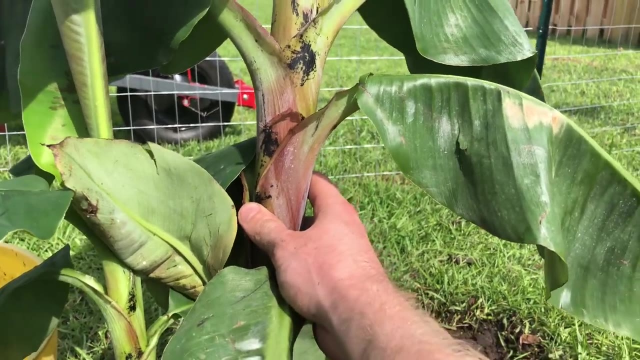 eventually the flower is gonna come out of here like a normal leaf. it's gonna bend over and you're gonna have fruit start forming on the actual stalk of the banana tree that starts bending over and then, once this tree fruits, it will die. so you can just go ahead and chop it down, get rid of it, but they continuously. 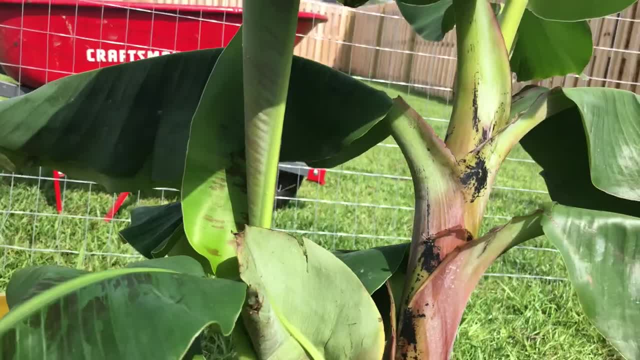 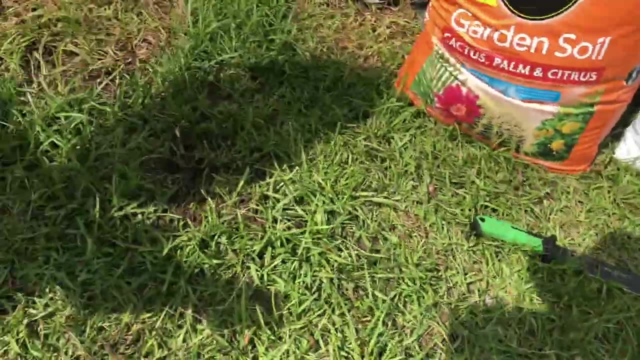 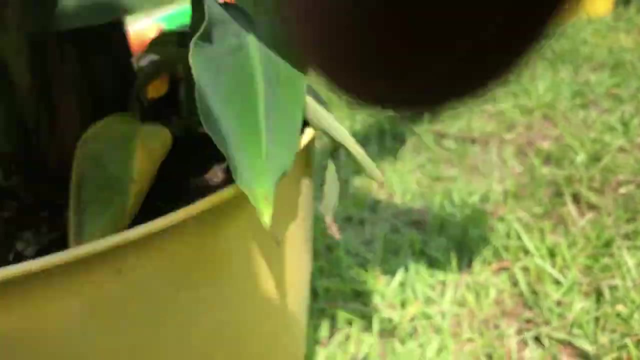 shoot off these little banana trees that come out from the same root ball down and we call these pups. and let's see, this other one has one too. yep, here's a. here's a little small one right here, there's actually looks like there's another one over here too. so one, two. 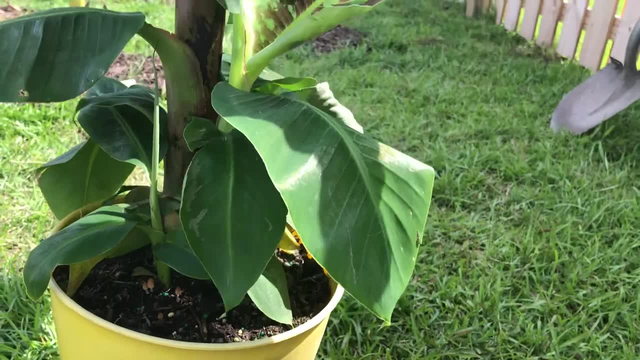 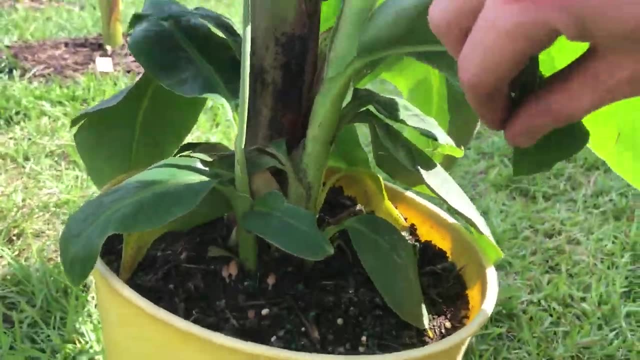 uh, three. actually, this one's got three coming off: this one and, uh, these are a little small. if you want them to live, you probably want to wait a little longer before you cut these off, but this one's over here. this one's so big it's ready to be one of its own. 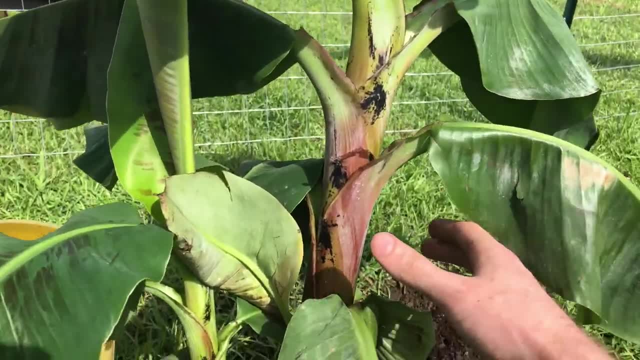 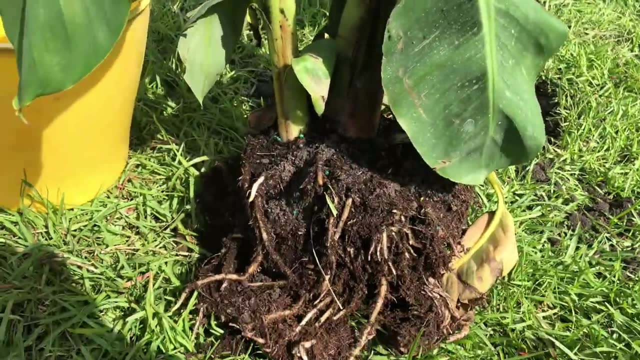 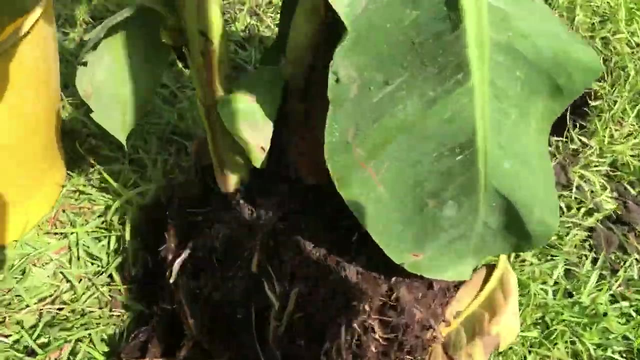 and it's actually so big that it's draining a lot of nutrients from this main banana stalk. so we're going to go ahead and cut it off, super simple, because it's this small. so we're going to take shovel, we're just going to take this right here. 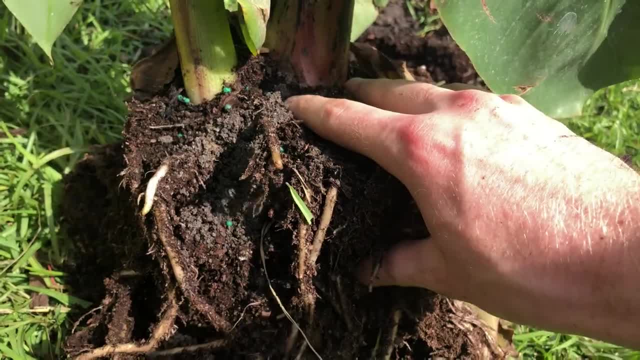 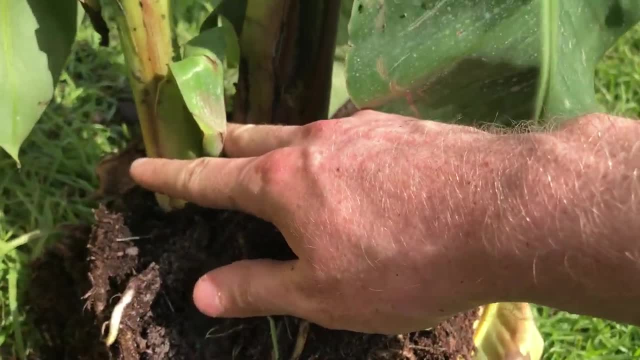 right in between. as you can see, they both come from the main root ball, the same root ball. so what you want to do is make sure you don't cut. don't cut right here or up here, or even wait on here. you want to go straight down and almost. 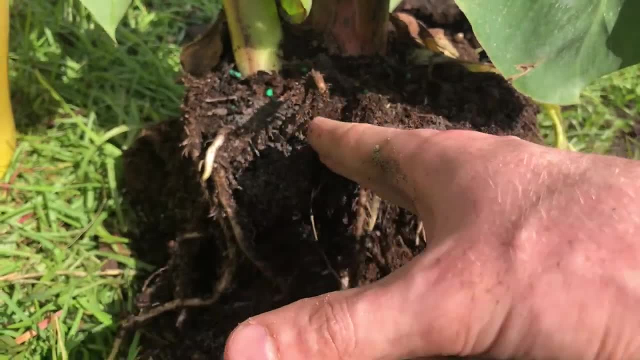 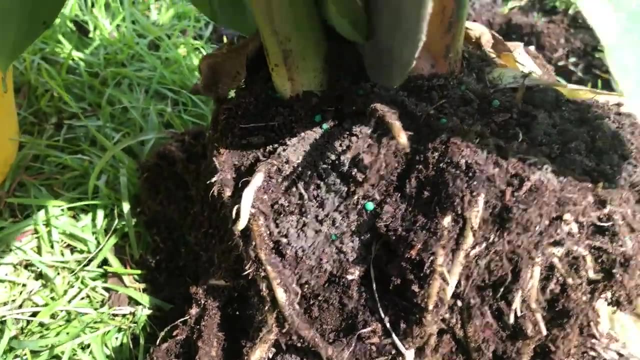 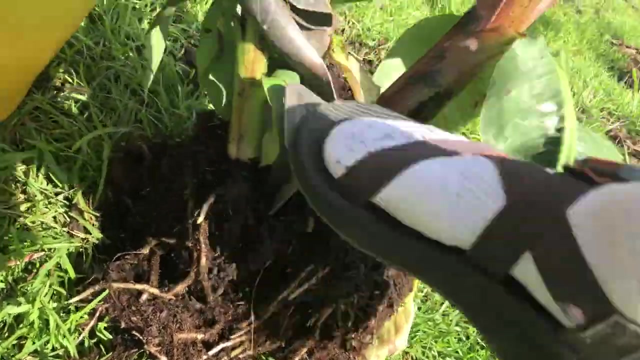 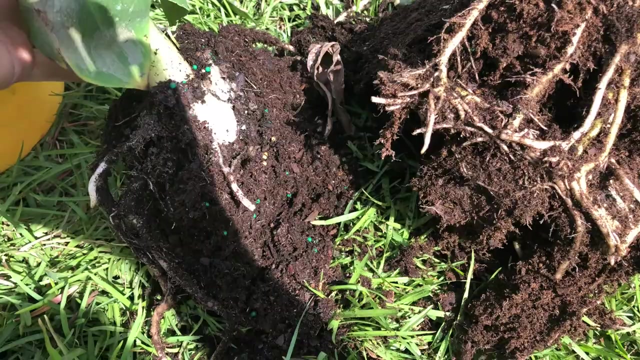 in a little bit, because you have to get some of this root ball with the pup, otherwise it will die. so we're gonna stick right in there and angle it back towards the banana tree a little bit and then break it off right there. all right, as you can see, look at all these great roots that came with this. 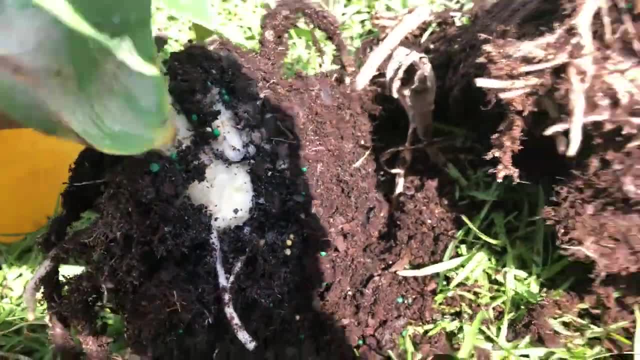 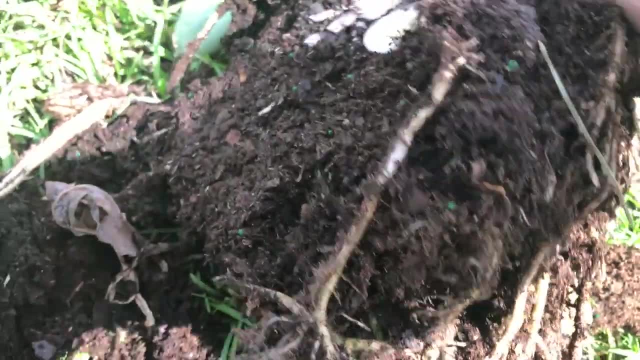 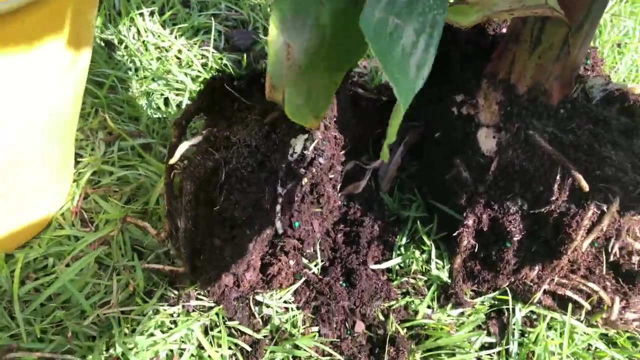 and then we broke up the main quorum just a little bit, where this guy still has the majority of it over here. so this guy's still going to continue to grow super healthy, but now so will this one. now we just have two dwarf cavendish now. 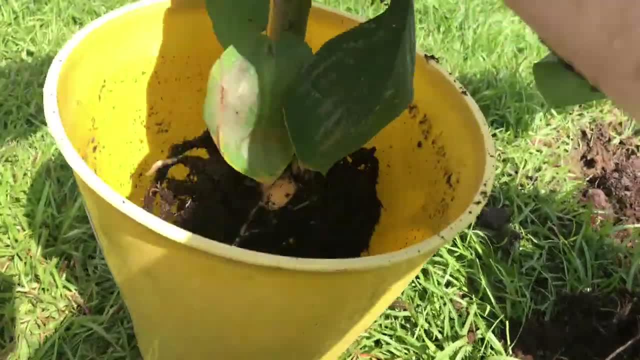 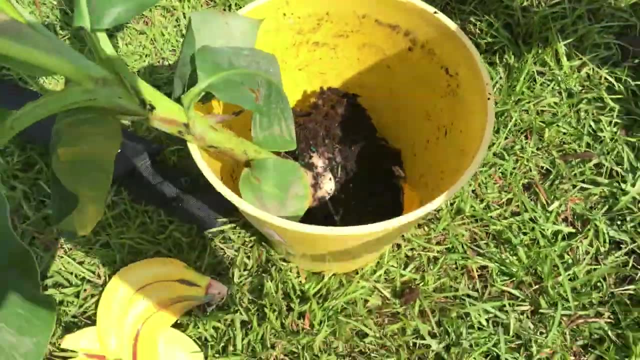 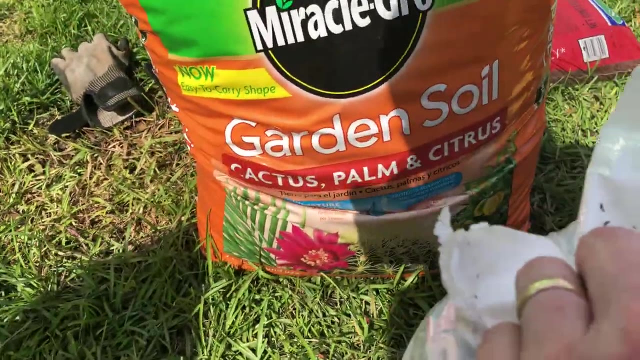 so we're gonna go ahead and put this guy in the pot of its own and, just like my video on how to plant a banana tree, we're gonna add a little bit of compost, and then i got some palm and citrus garden soil, so we're gonna go ahead and put those in. 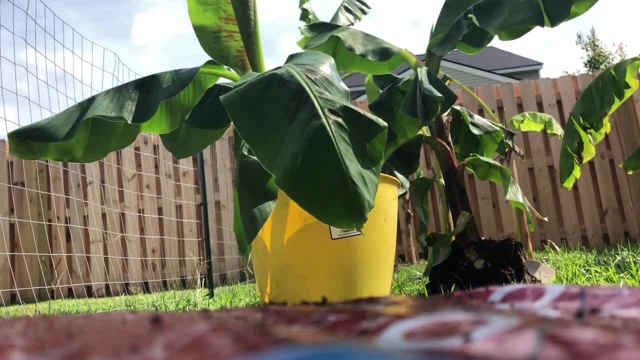 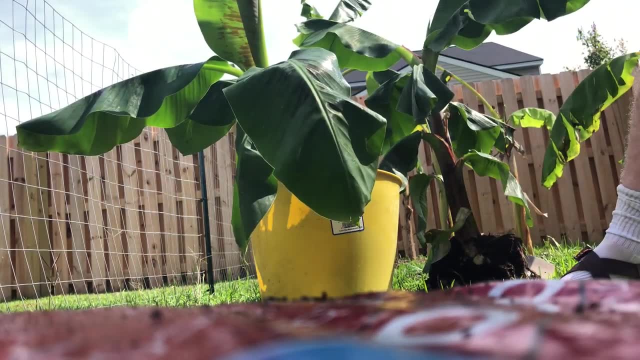 let's set this up right here, and it looks like we're almost done. we're gonna go ahead and put those in the pot and i'm gonna flip this over and you're gonna see it's all fully planted. and you're gonna see it's all planted. 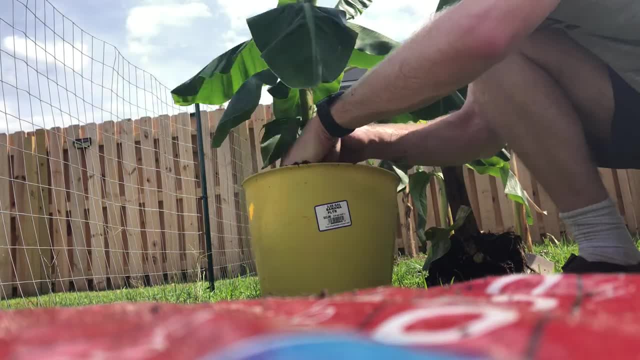 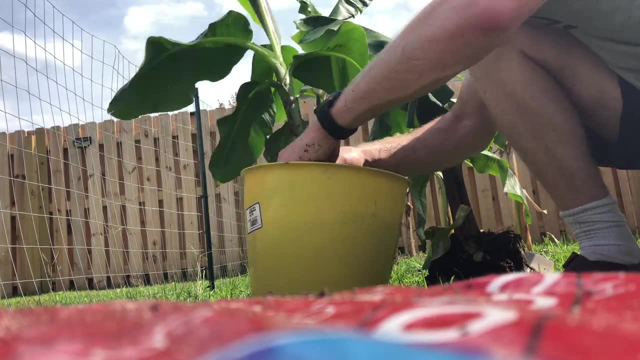 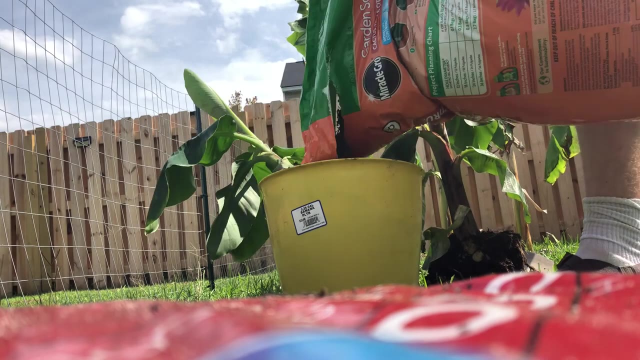 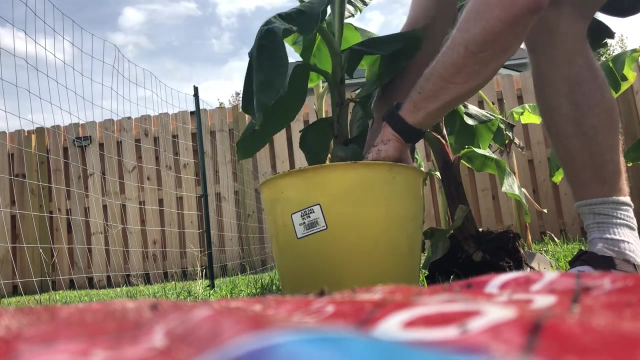 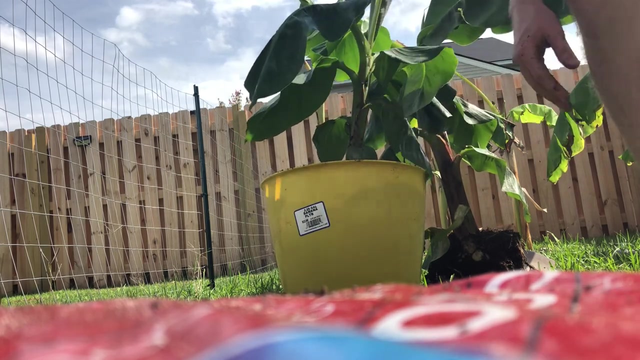 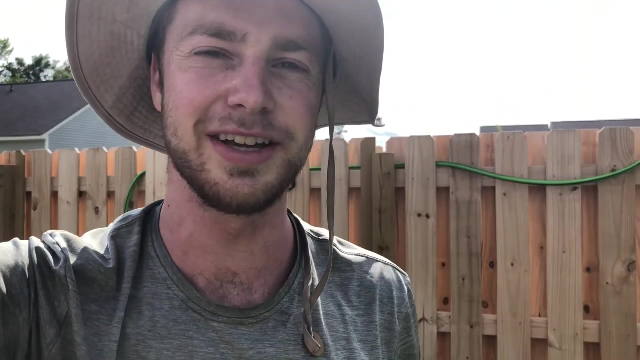 we're gonna get a little bit of water. let's take a quick look at the bedding. it looks like we're almost ready, or maybe not, i don't know. let's do this. all right, that guy's good to go and we're going to send him off to atlanta and he should live and. 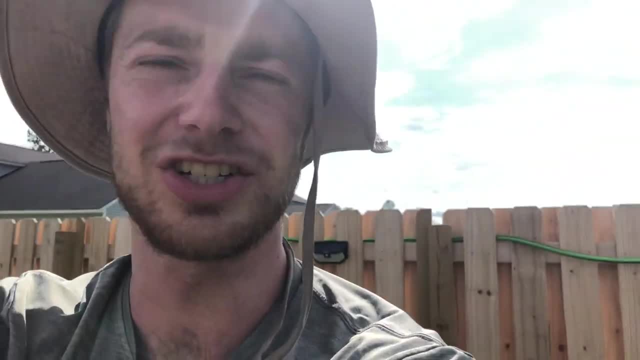 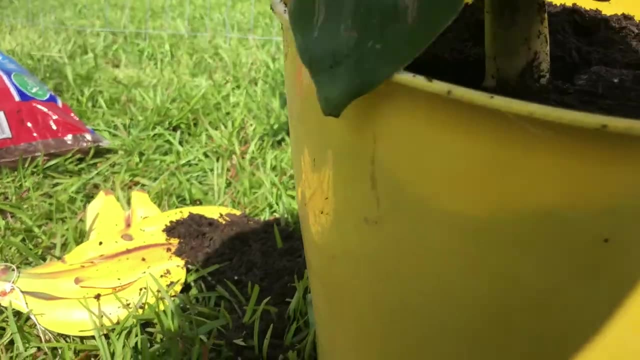 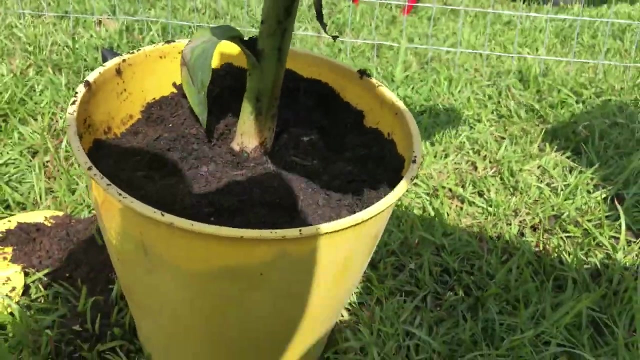 fruit, some bananas in a couple, uh, couple years, maybe next year, probably a couple years though. um, right down in there leaning a little bit, we're gonna have to prop them up, maybe add a little bit of mulch as well, but this guy's ready to go and you can keep doing that for.